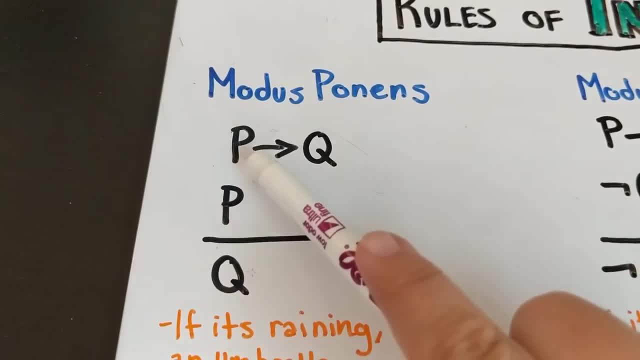 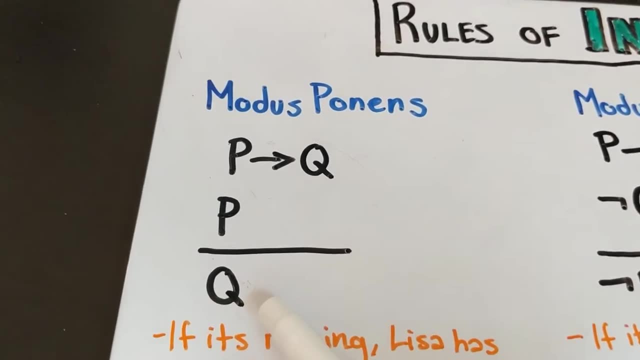 and this is the rule that says: if you have in your model P, then Q is true and you know that P is true, you can conclude that Q is true. So if you have in your model P, then Q is true and you know that P is true, you can conclude that Q is true. 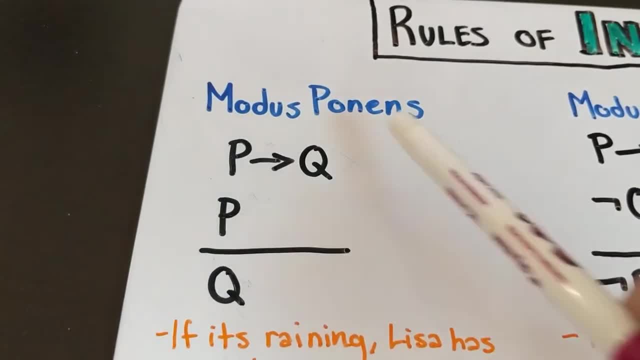 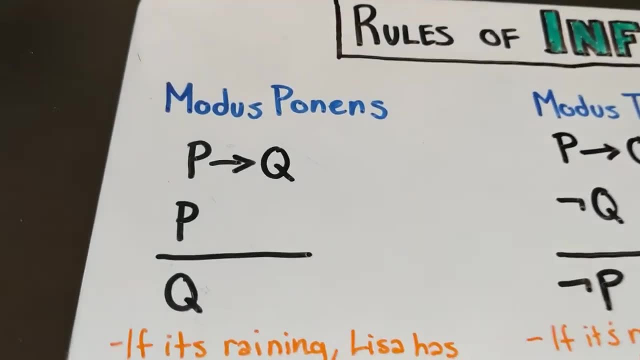 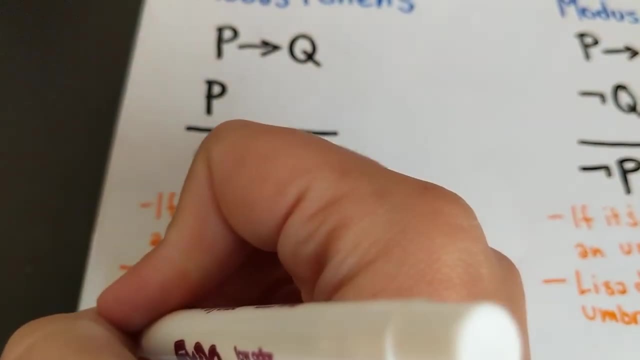 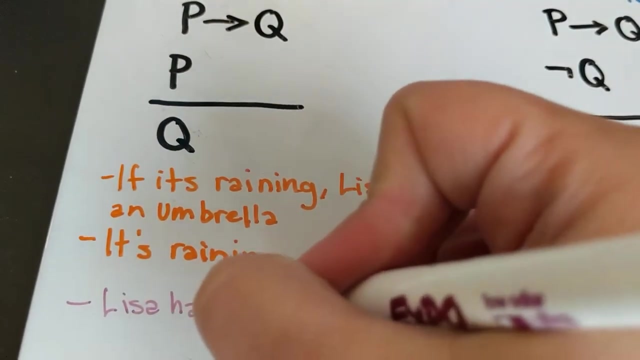 This is basically just more of the, the definition of if-then right. It's the definition of this symbol. So, for example, if you say, if it's raining, Lisa has an umbrella, you know it's raining. you can conclude: Lisa has an umbrella. 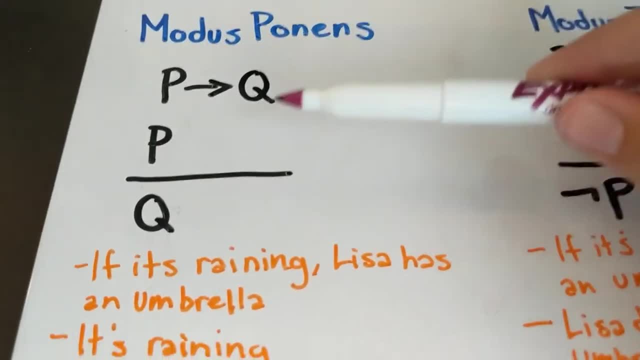 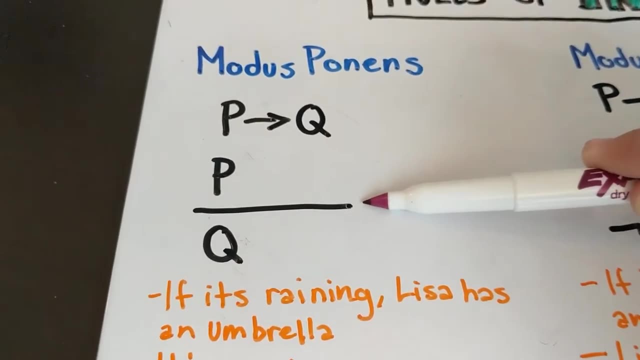 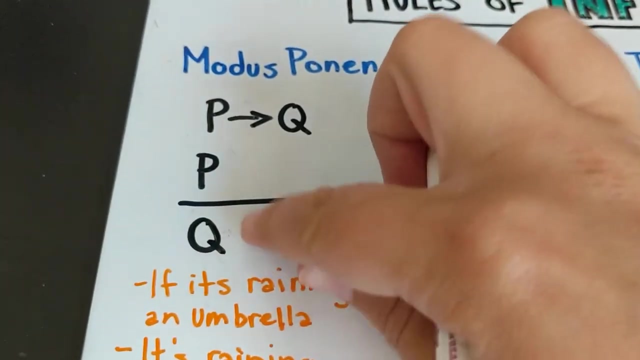 That's your conclusion, right? And when we write out these rules, we take: this is this is a given, this is another given, and then you apply a rule, you put a line where we apply modus ponens, and this is your conclusion. This is your inference, right? Okay, our next one is called modus. 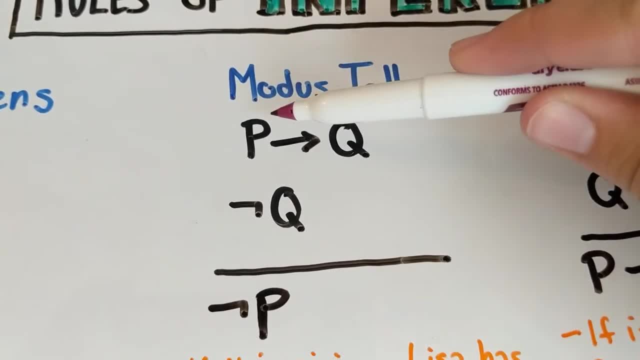 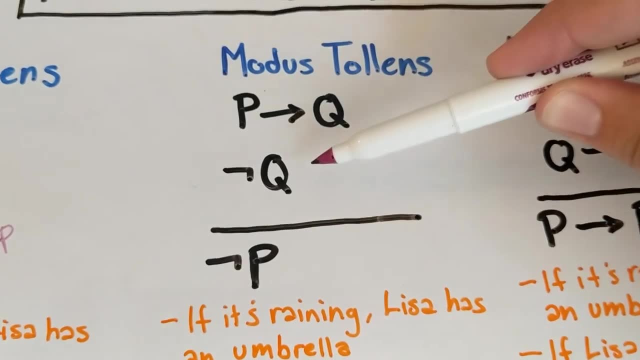 tollens and this one. in this rule we say: if we have in our, in our model, that P, then Q is true. So if we have in our, in our model, that P, then Q is true. And we know that Q is not true, right, So not Q is in our model, right? Not Q is. 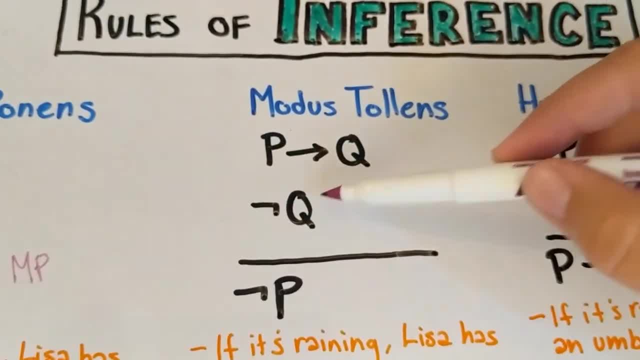 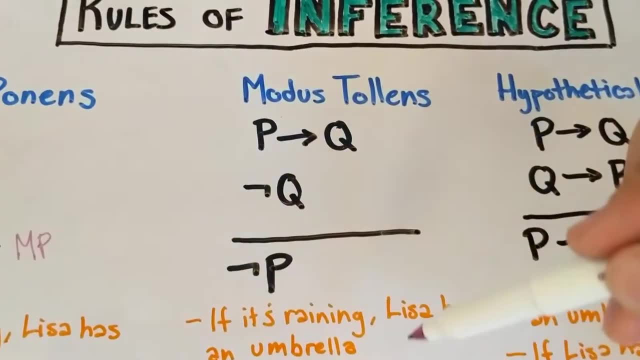 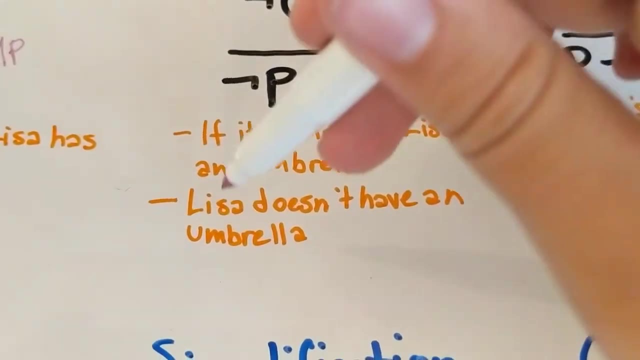 true, So P, Q is false, right. Then we can conclude that P is also not true. So this one is a little bit less intuitive. but once you see an example with words, this makes a lot more sense. If it's raining, Lisa has an umbrella, and we know. 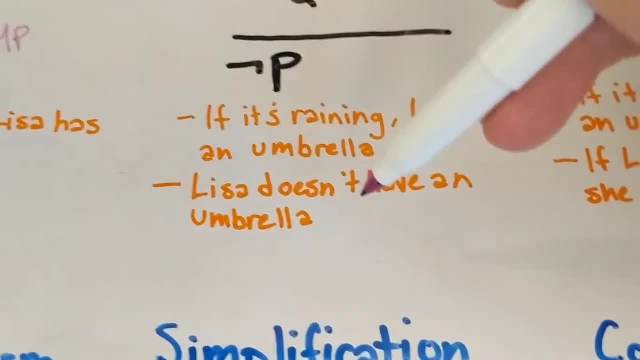 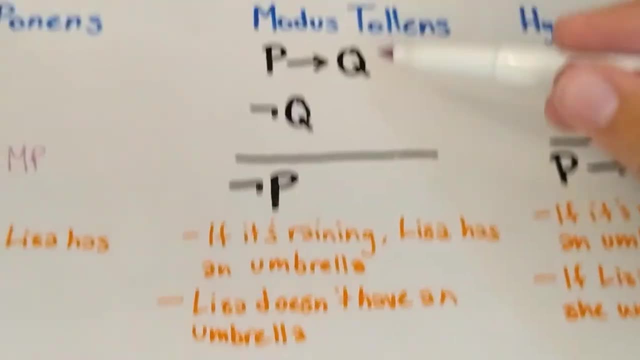 that Lisa doesn't have an umbrella, right? So we know that it must not be raining, Right? Because if she, if she, didn't have an umbrella and it was raining, then this could not be true, right? Does that make sense? So so this is mostly about 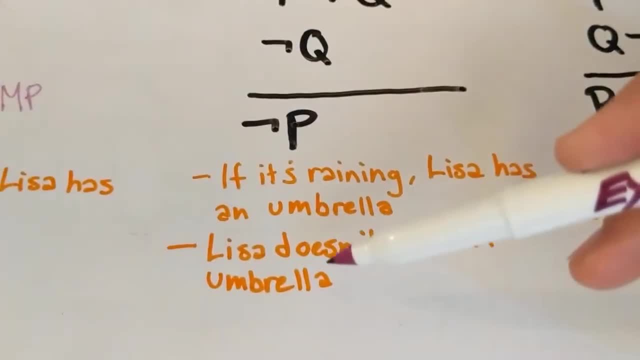 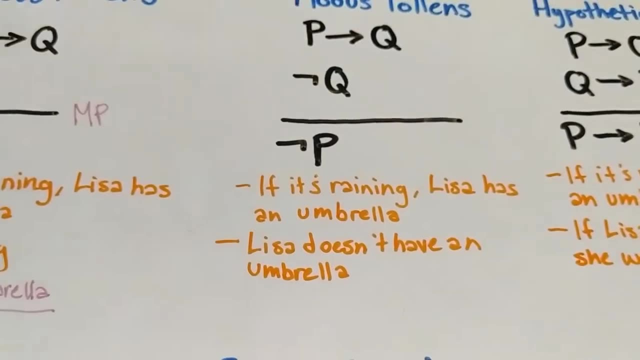 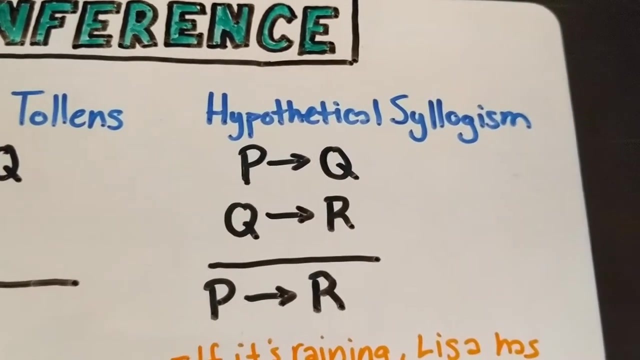 eliminating the one case where, where this, this symbol would be false, right, Yeah, All right. our next is is something that's not exactly something we've seen before, but this is the hypothetical syllogism. This says that if P, then Q is. 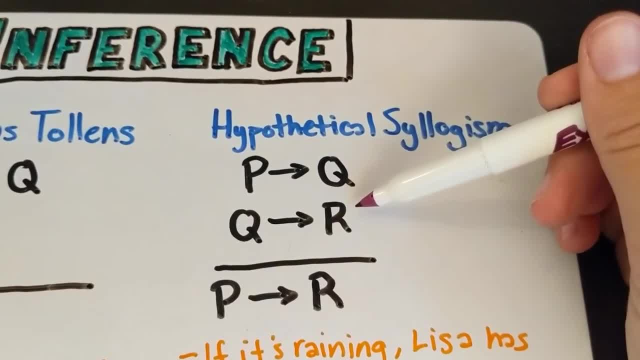 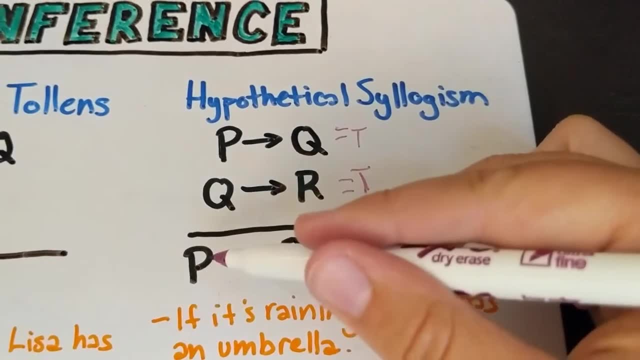 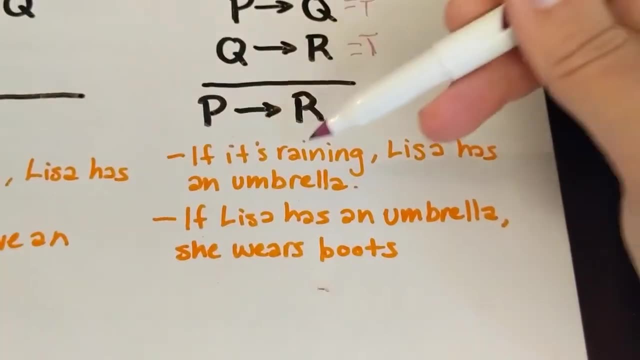 in our model and Q then R is in our model. if these are both true, right, These are both true statements, then we know that P then R also has to be true. So, for example, if we have the statement if it's raining, Lisa has an umbrella, and we 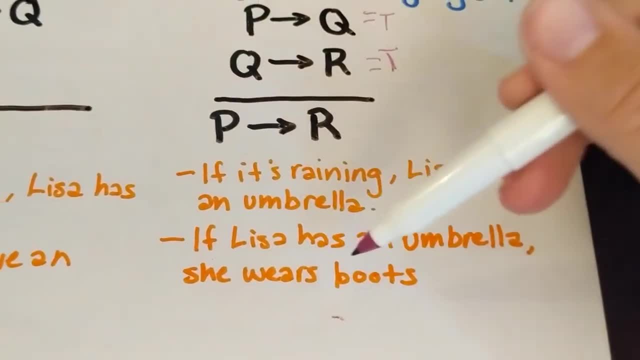 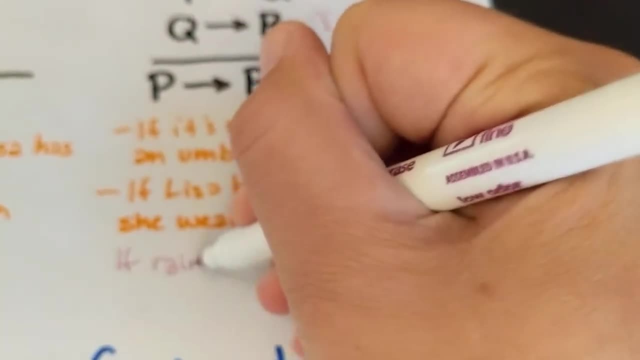 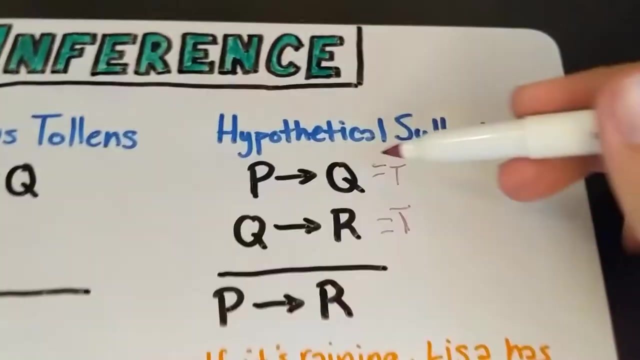 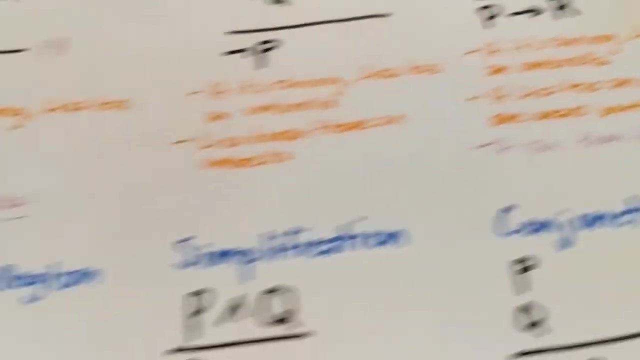 also have the statement: if Lisa has an umbrella, she wears boots, right. We can then conclude: if it's raining, then boots right. As long as we know that both these statements are true, we can conclude that this statement is also true, right? Okay, Our next one is: 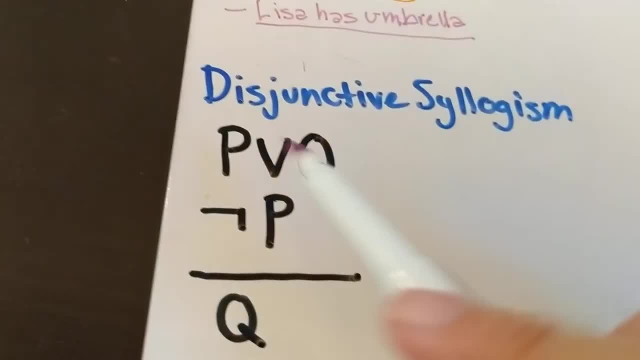 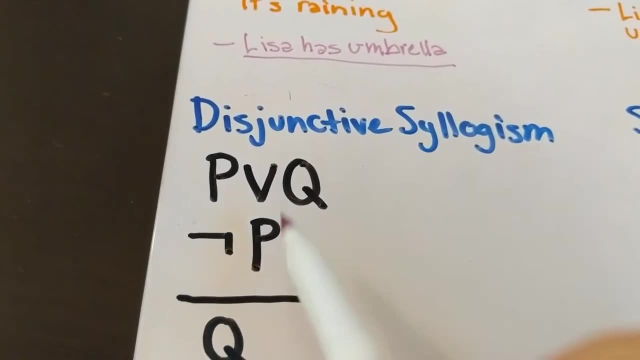 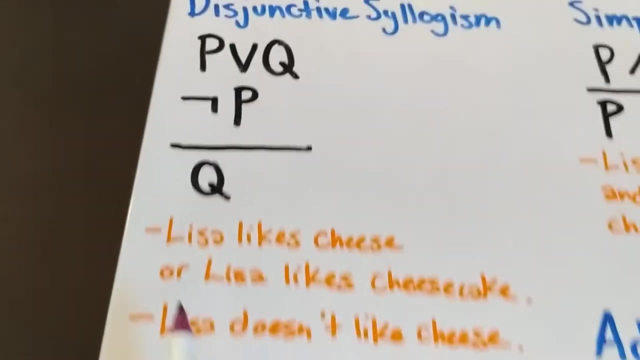 called the disjunctive syllogism. This says that if you know that P or Q is true in your model and you know that not P is true in your model- meaning that P is false in your model- then you can conclude that Q must be true. This makes a lot of sense if you 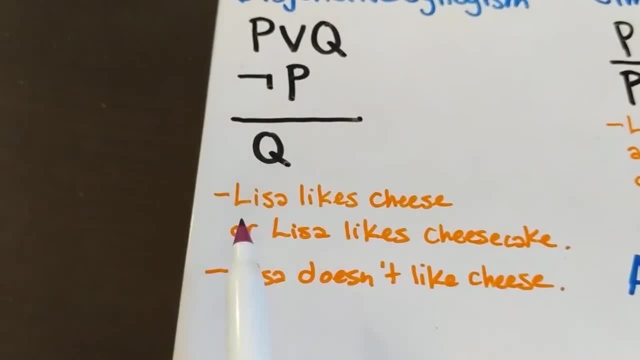 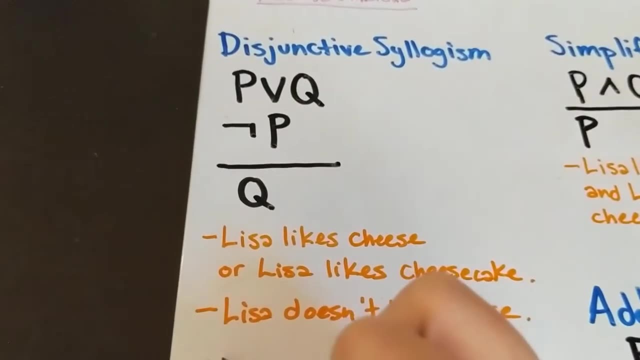 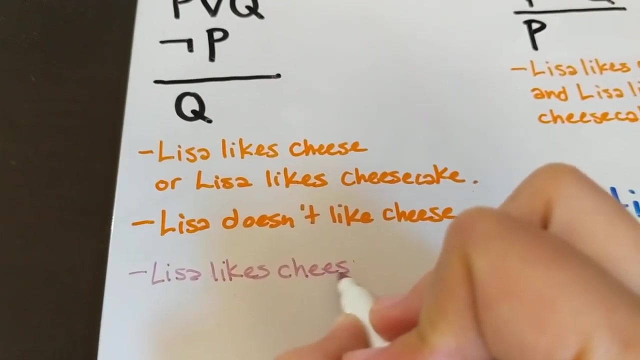 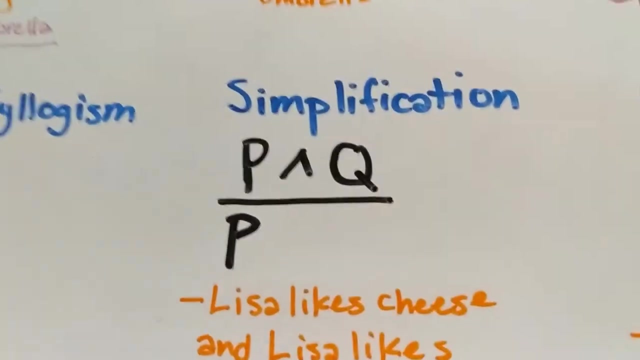 look at the example. So Lisa likes cheese, or Lisa likes cheesecake, Lisa doesn't like cheese. Since we know this was true, we have to know that Lisa likes cheesecake. Here's our conclusion, right? So yeah, Okay. So they're all true then. So you know that p and q is true, okay? And if they're? 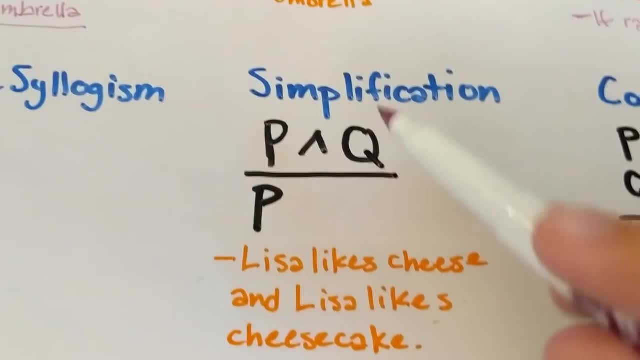 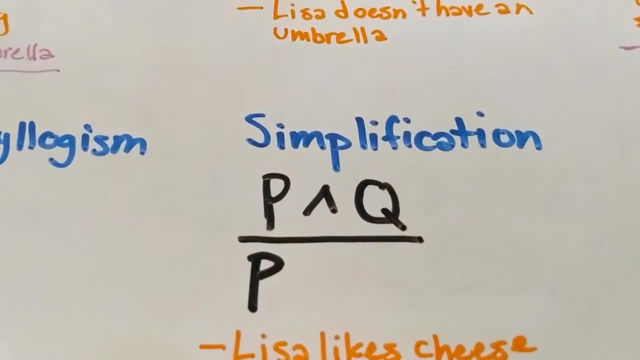 both true, then you have to, like you know, help her out a bit with proofs. Okay, so the last part of our next really cool question is: I don't know if this shift in Hebrew Project was the good question or not, but it's. it's got lots. 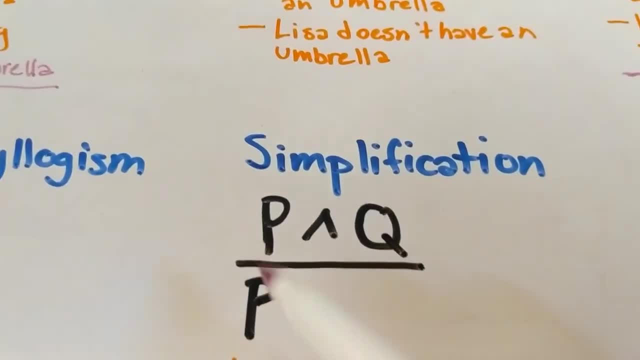 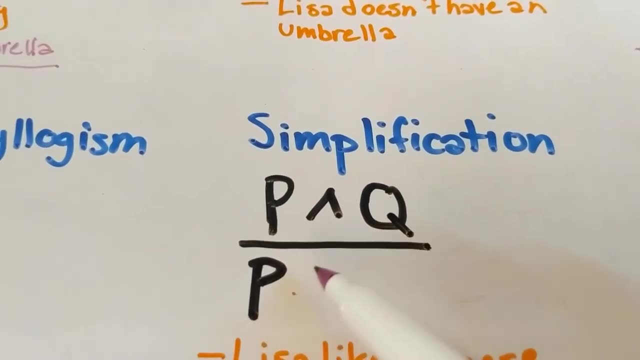 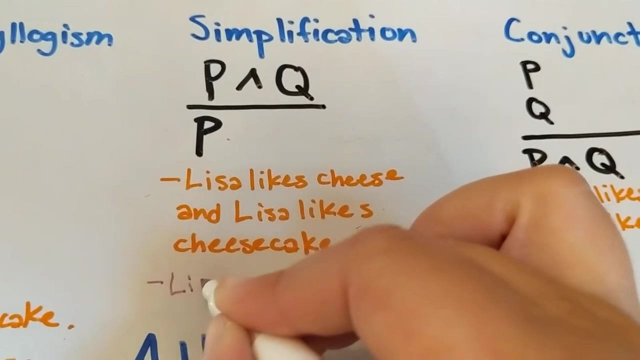 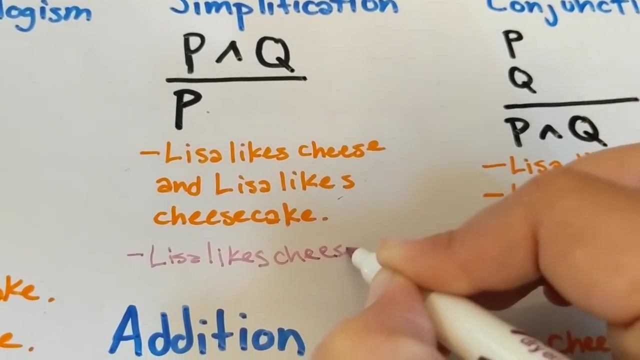 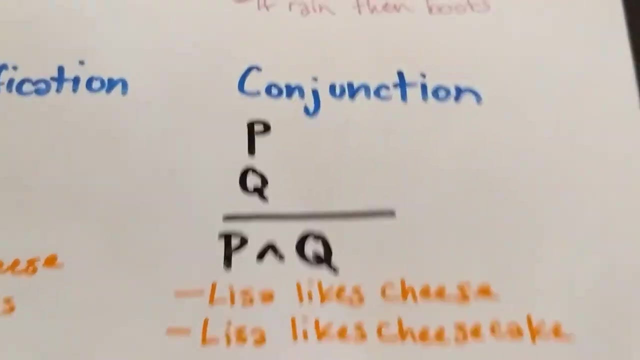 of of non- quotable things going on in here. otherils, though, Okay, And so cheesecake is true. you can conclude that Lisa likes cheese must also be true, right? So this allows you to shrink your statements. Conjunction allows you to build statements, So if you know,